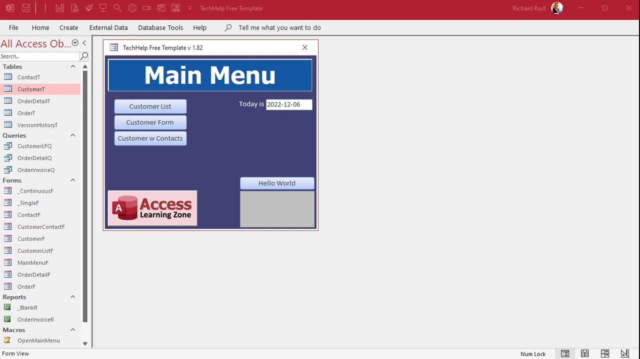 Fortunately, there is a built-in function called IsDate that we can use, And you can use it to determine if a particular date is a valid date or not. So if someone types something in and you want to know if it's a date, you can ask IsDate. 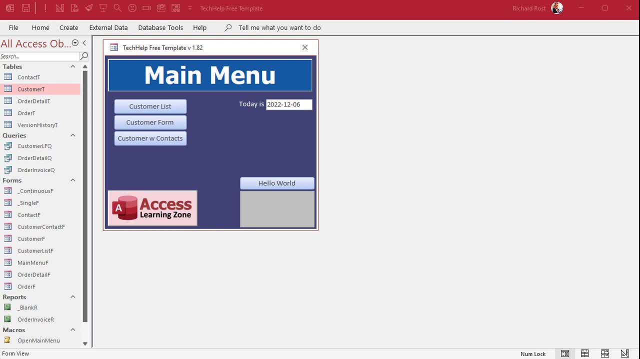 How do we use this to determine leap years? Well, we can make a fake date, which would be February 29th of whatever particular year, and then ask: IsDate, is that a valid date? And if it says no, then 229, 1987 doesn't exist, so it's not a valid date. 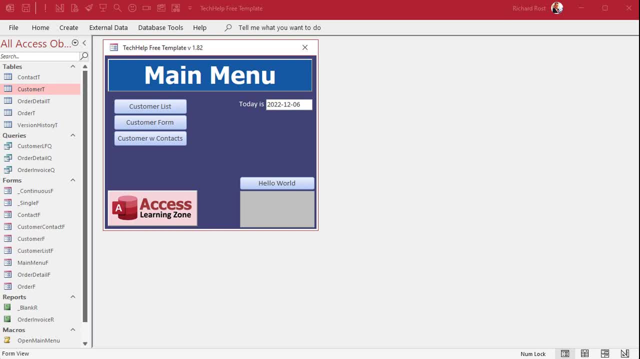 And IsDate can tell you if that date is valid. So it's a tool for determining how leap years work. So let's see how this works in the database. This is my Tech Help free template. You can download a free copy of this off my website if you want to. 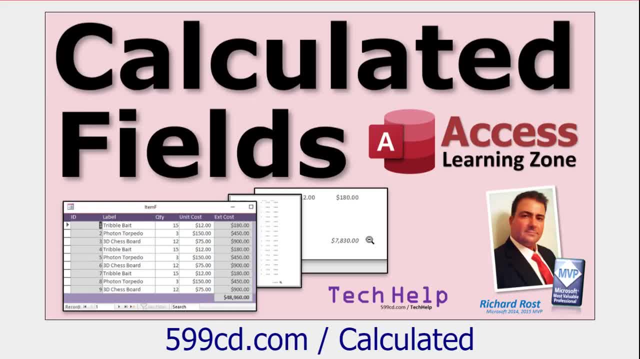 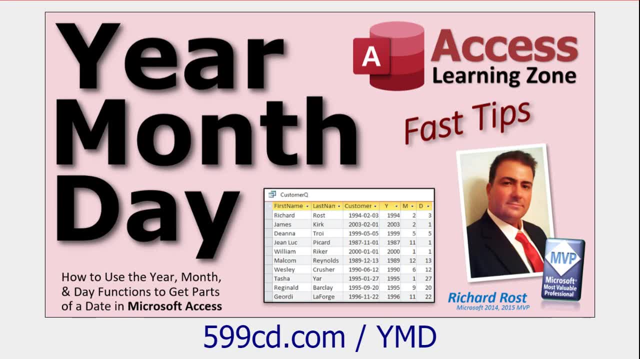 A couple of prerequisites for you. first, If you don't know how to use calculated fields and queries, go watch this. You should also know how to use the year, month and day functions. We're going to use the year function to pull the year value out of any given date. 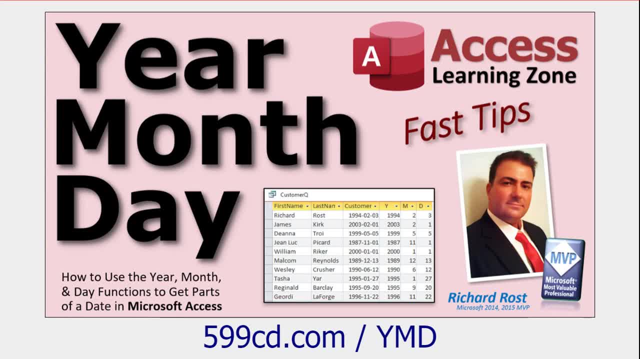 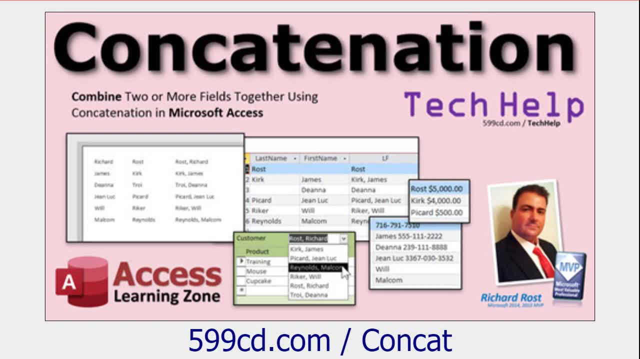 So if I tell it January 1st 1980, it'll give me the 1980 part. And finally, we're going to use a little string concatenation, that's putting two strings together, to use this little trick with IsDate. 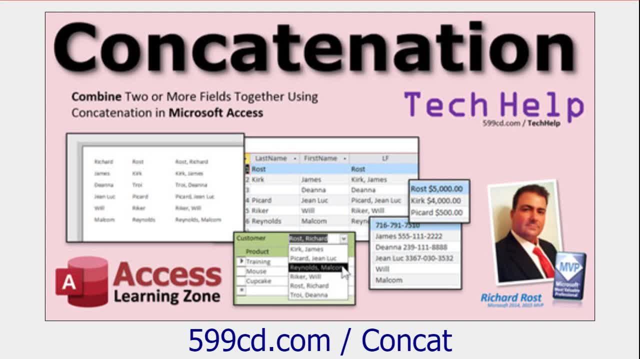 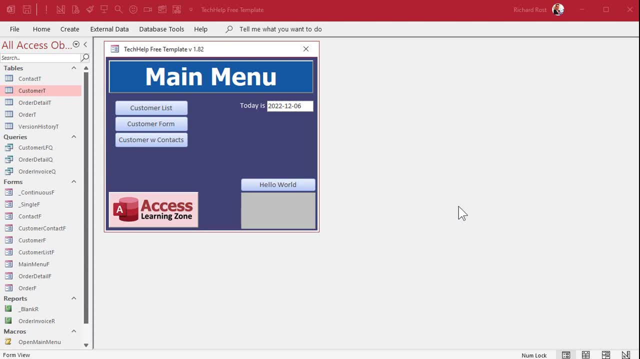 So if you don't know anything about those three topics, go watch those videos first. You'll find links to them down below in the description under the video window. Go watch those and then come on back. Okay, in my customer table I've got a field with a whole bunch of dates in it. 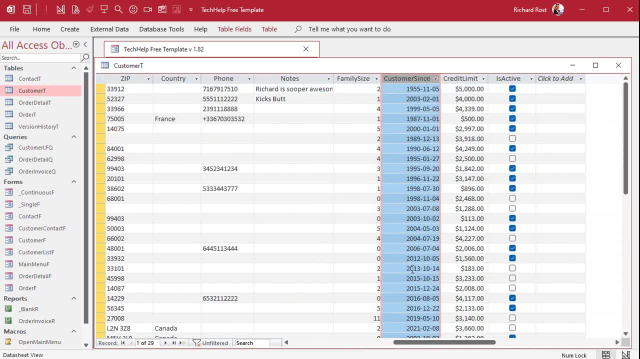 Where is that? Let's see right here My customer sense field. So we'll use that as the date. we're trying to determine if that year is a leap year And of course I've got a field with a whole bunch of dates in it. 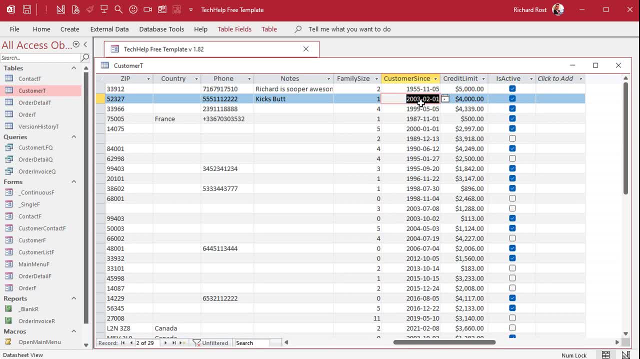 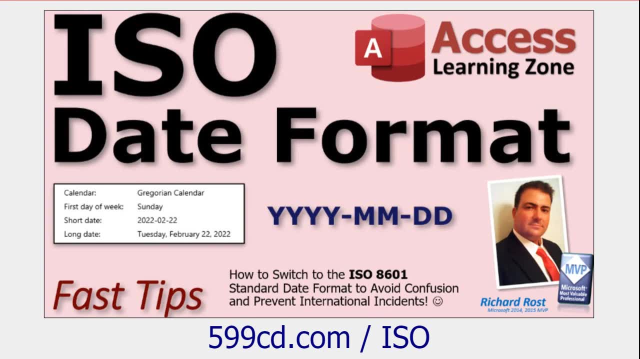 I use the ISO date standard, which is year, month, day. It's universally accepted. I've got students all over the world. There's one more video for you to go watch if you're interested in that. This way, we're all on the same page when it comes to a date format. 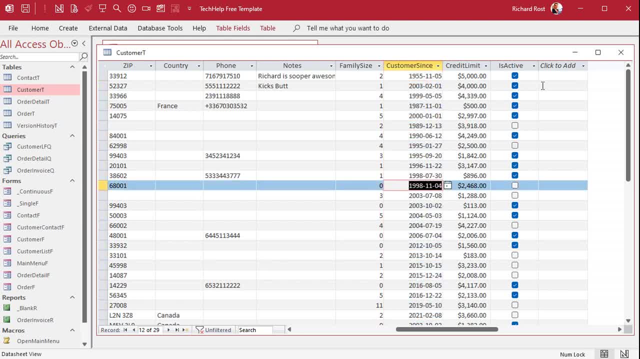 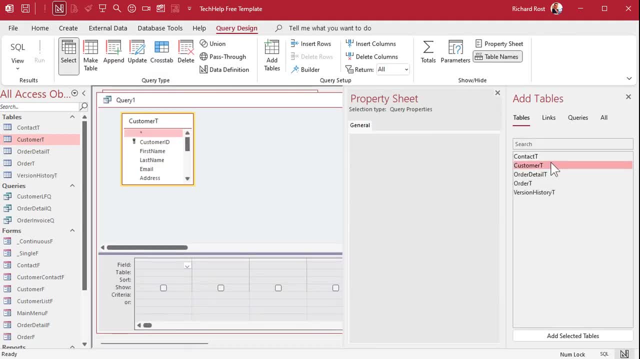 All right. so I want to see if that date, for example, happens to fall on a leap year. So let's make a query, Create Query design And I'll bring in my customer table And I'll close these little guys down. 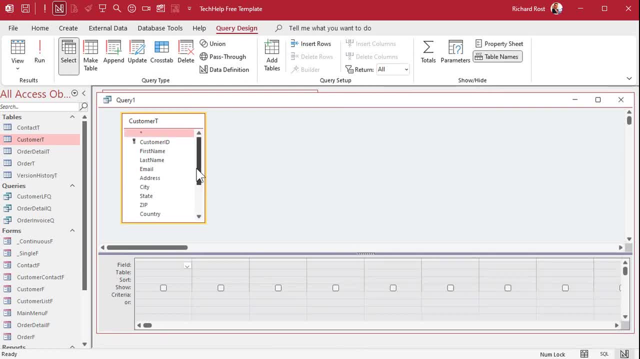 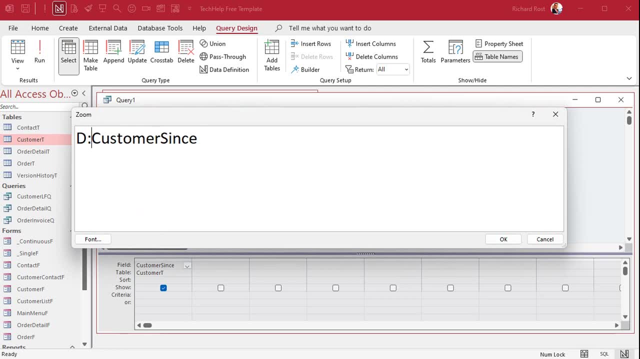 We don't need those. All right, let's find that customer sense field. Bring that down here Now. I don't want to have to keep referring to customer sense, So I'm going to alias that guy. I'm going to say D colon. 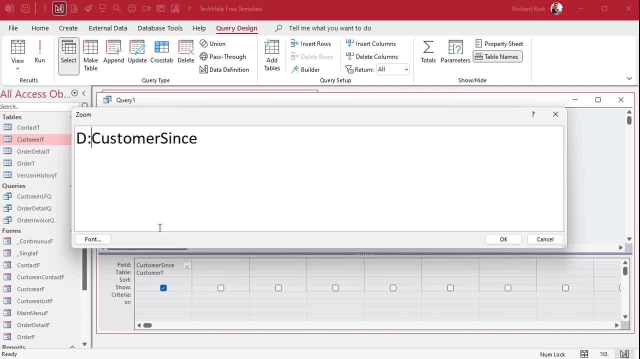 In other words, I'm going to call customer sense D. This is a shorthand. It's easier to type in all my things and all my other calculations here. Just refer to it as D And you can plug any other value that you want in there. 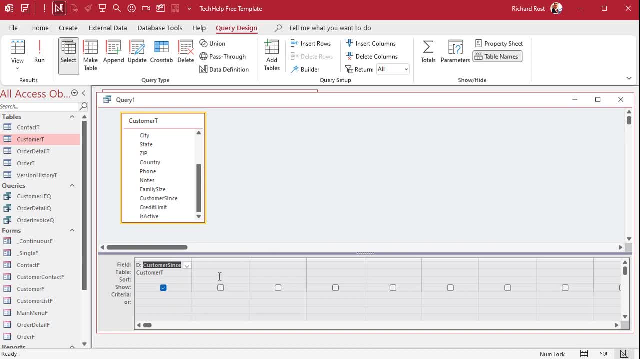 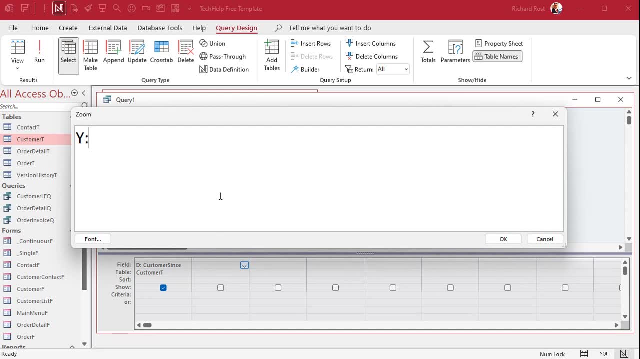 Now I want to figure out what the year of that date value is. So in the next field over here, shift F2, zoom in. I'm going to call another variable, Y, And that's going to be the year of D. 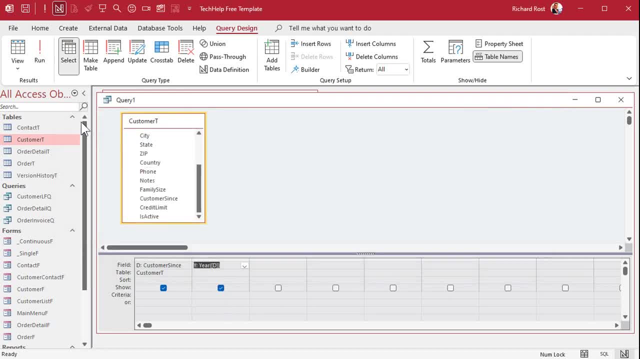 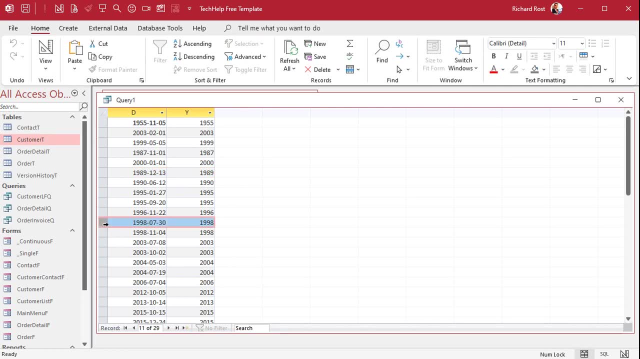 All right, so take D, give me its year and bam, there you go, So that guy there falls in 1989.. All right, there's a number representing that year. Easy enough so far. right, That's the easy stuff. 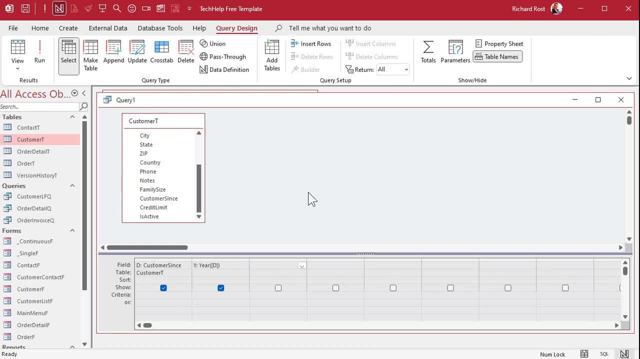 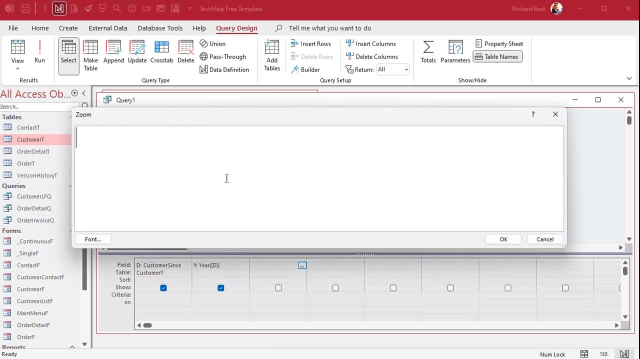 Okay, next up, we're going to use string concatenation to build a date that's going to be this year, followed by February 29th. Okay, now, again, I'm using the ISO date standard, So I'm going to call it D2, where R2 is, I don't know. 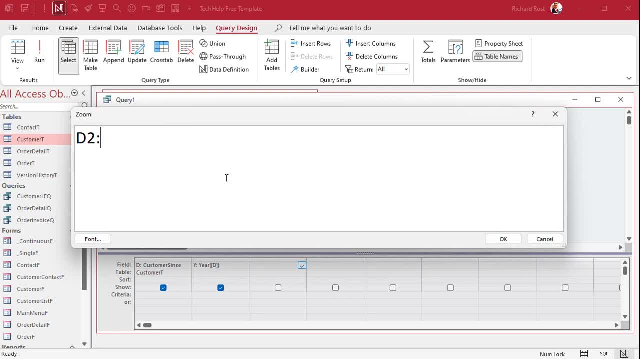 There's D2.. There's D2.. A little nerdy Star Wars joke for you. Okay, so this is going to be Y, that'll be 1990 or whatever ampersand. so string concatenation. quote: dash 02-29.. 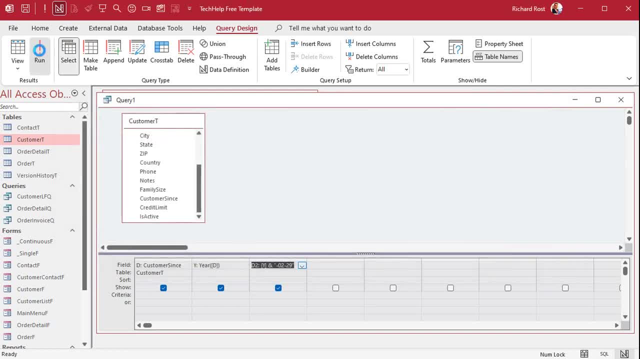 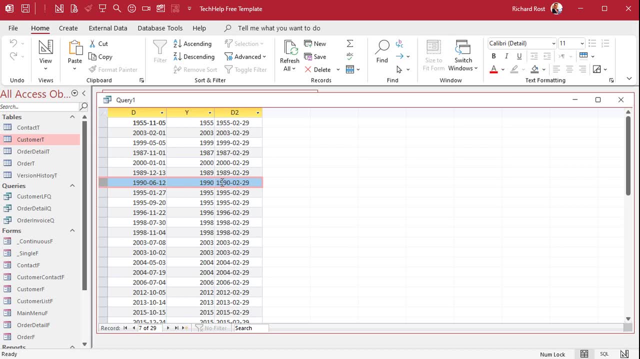 Okay, hit, all right, hit, okay and run it, and there's your fake date, right. So there, for example, 1990, right, 1990, June 12th. We got 1990, February 29th of every year in this. 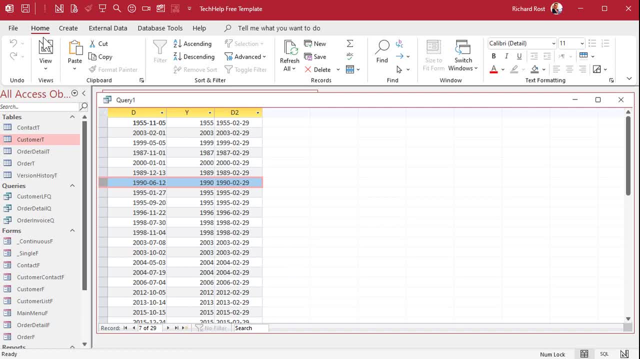 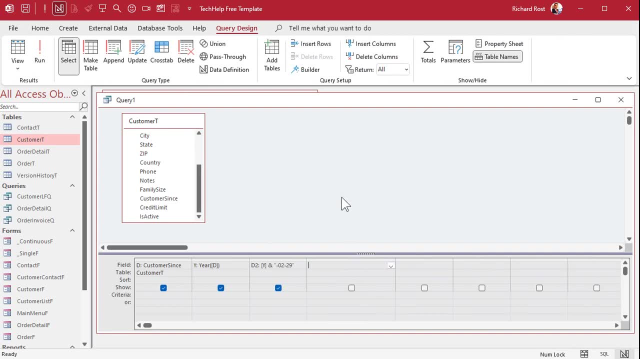 Okay and yes, just for the curious people, this will also work if you want to use your regional date format and you don't want to stick to the ISO dates. For example, if I said it was, let's say, 2-29-and-Y, all right, this will also work. 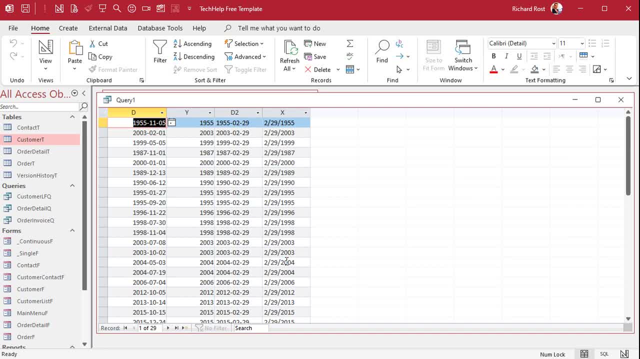 Like I'm in the US. so if you want to use your local standard, you can do that too, But I'm ISO, so I'm going to stick with this one. Okay, all right, let's go to that. 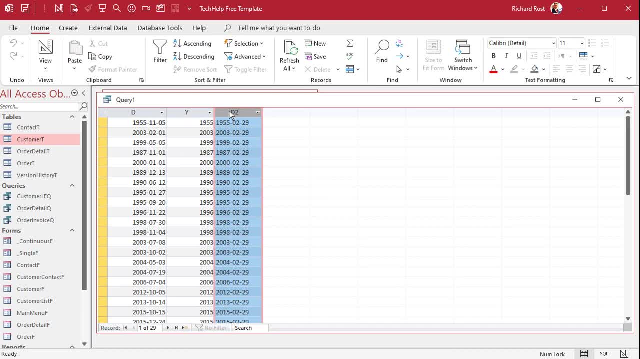 All right. so we've got a whole column full of fake dates here. Now the trick is to see, using is date, if that's a valid date. Also one more thing to notice: notice how these guys line up on the left side of the column. 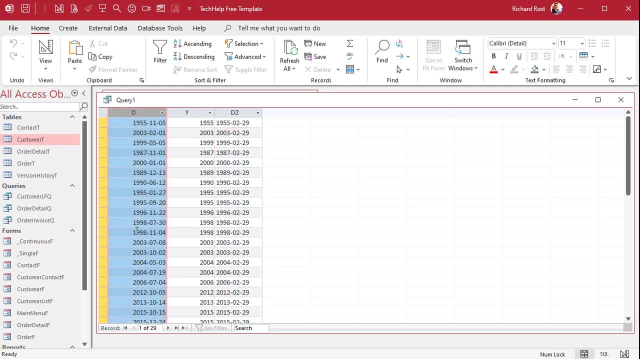 These guys line up on the right Numeric values which include dates, right currency numbers, date values. those are all numeric types versus text strings. all line up on the left side. That's one giveaway right there. You could tell that's a text value, okay. 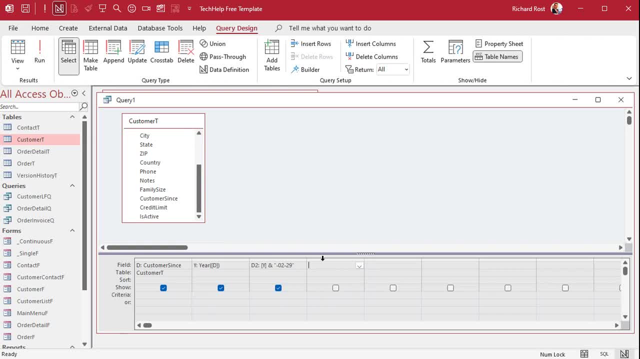 So the next step is to say: hey, is that a valid date? So we're going to call it isLeapHere. Let me zoom in again. isLeapHere colon. we're going to use the isDate function and put D2 in there. 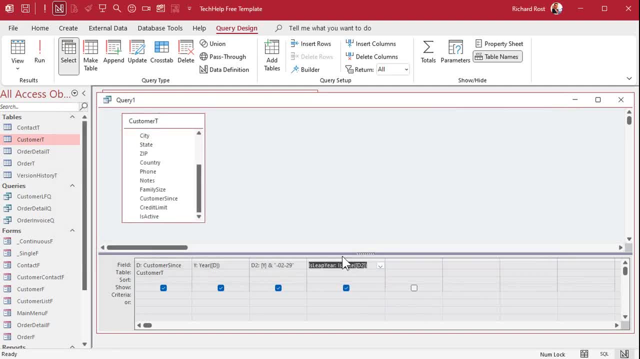 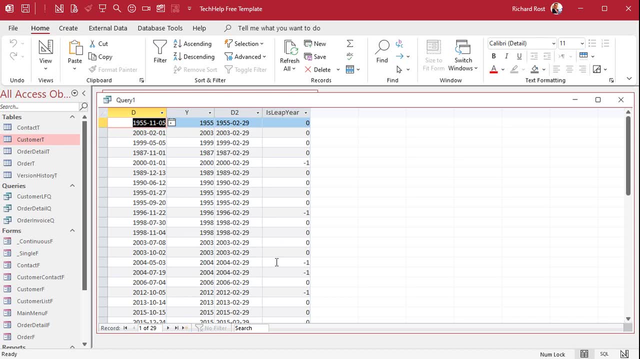 All right. so is that guy there next to it that we just built? is that a valid date? And now we'll run it. And there's a bunch of zeros, Zeros and minus ones. Remember, in Access, minus one is true or yes, zero is false. 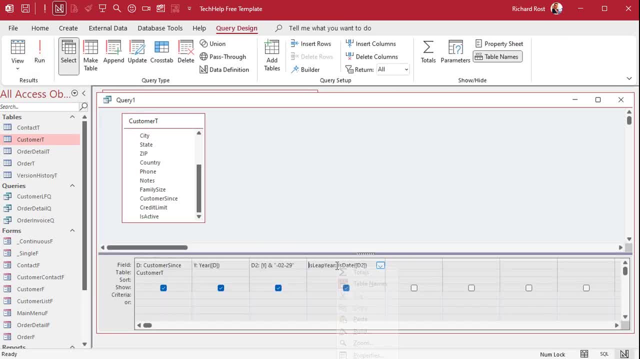 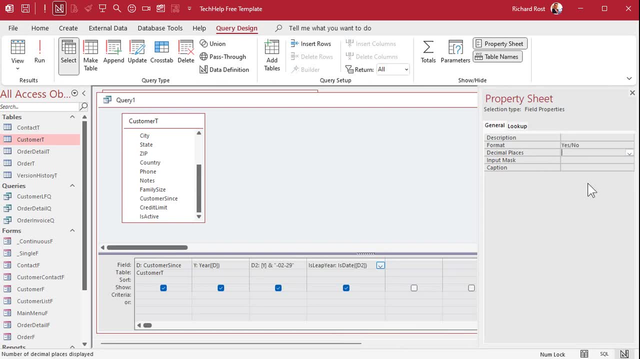 If you want to format that to show yes or no, you can right-click, go to Properties and then in Format you can put in here: yes, slash, no or true, slash, false or on slash off. 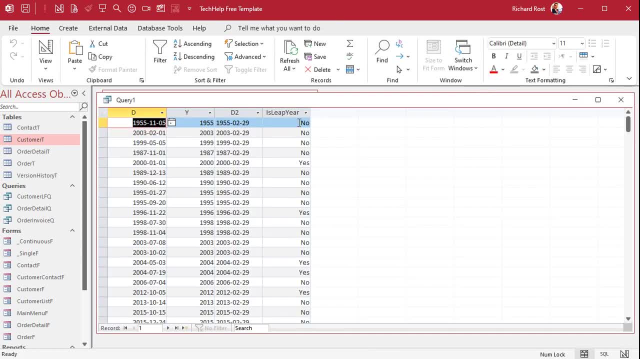 whatever you want, Lots of different formats are valid. Now, when I run it, I get yeses and nos And there you go. 2000 was a leap year. Remember that rule. It's different on those thousands years Because if it's divisible by four it is a leap year, unless it's divisible by 100, in which case it's not a leap year. 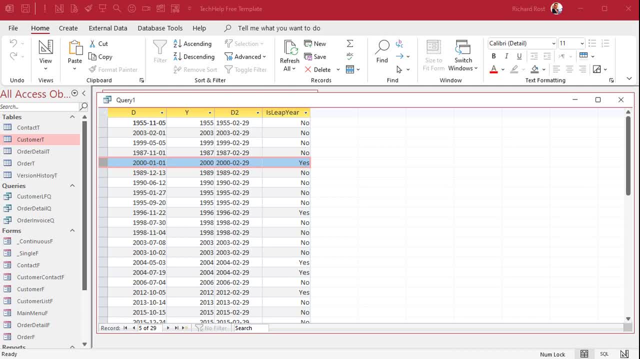 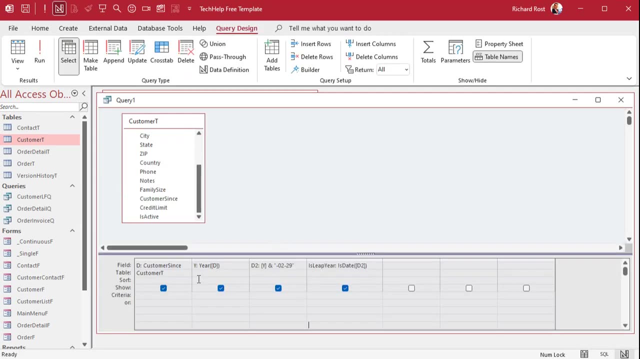 unless it's also divisible by 400, and then it is a leap year again. So, yeah, okay, Thank you for all the crazy date stuff, our fantastic calendar. Now you're probably saying to yourself self: is there an easier way to write all this than have that all in multiple steps like that? 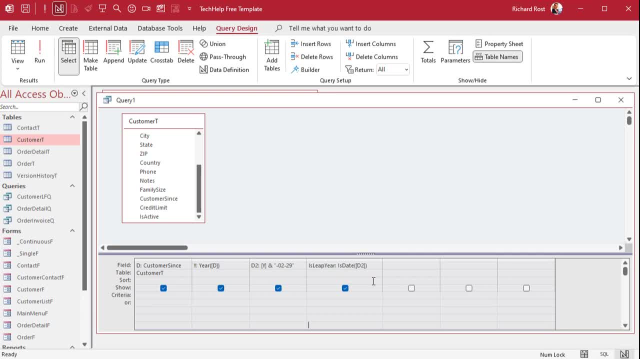 Yeah, of course. Of course, the multiple steps is what I show you when I'm teaching you how to do something, so you can see how I got to where I got to. all right, instead of just giving you one big function and saying, there, it is right. 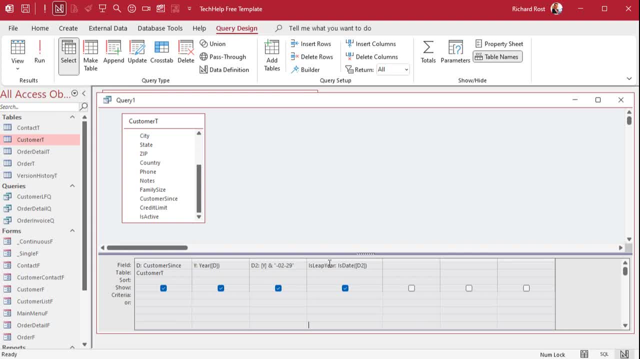 This way. you see, we've got to get the year, we've got to make a date out of it, we've got to check if that date's valid. But if you want to boil this down into one statement, you certainly can. It may make it harder for other people to read or for you in the future to figure out what you were doing. 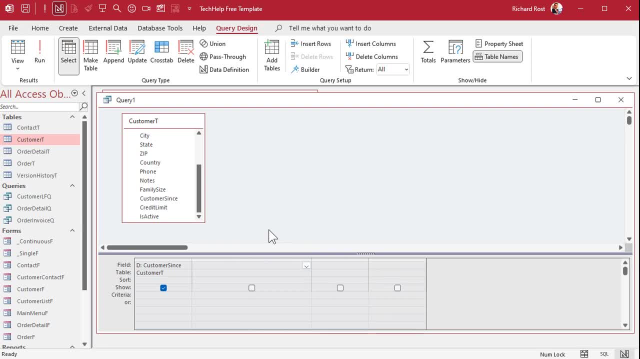 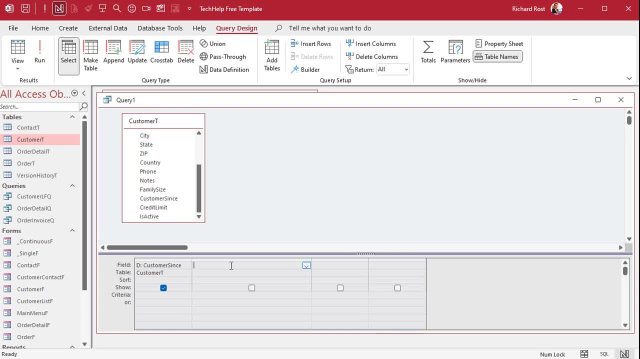 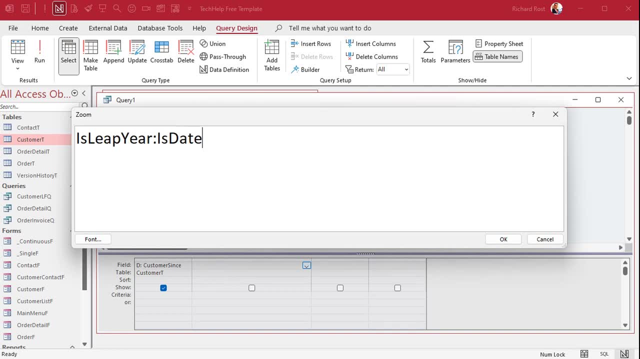 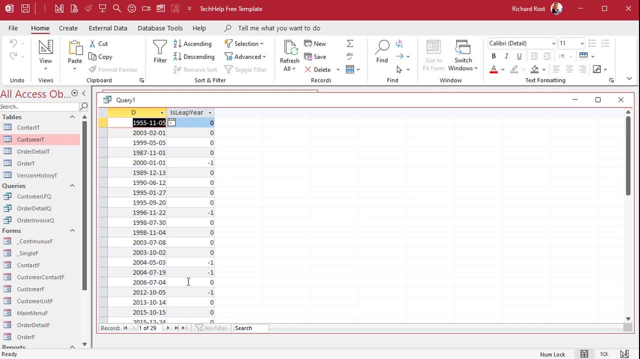 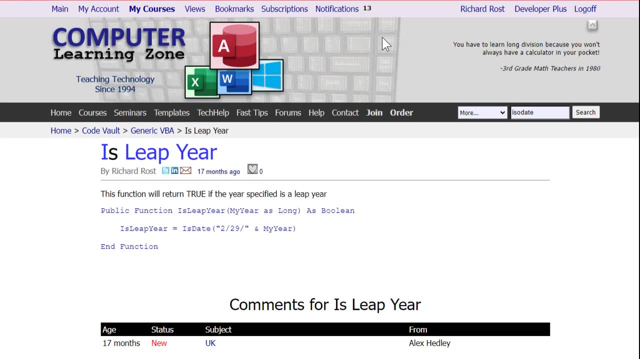 Hit okay, run it, and there you go. Formatted is yes, no. if you want to, and there's your final function. Can you use this in VS? Can you use this in VS b code? certainly you can. here i wrote a little function for it right there. very similar same. 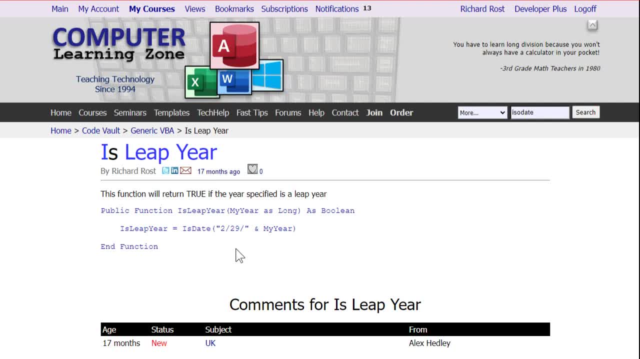 thing. this one's in the old us format. it's 17 months old, so i did this before i switched to iso, but it works either way, okay, uh, public function is leap year. you send it a year like you'll send it 1980, and it will return a true false value if that date is a valid date, if it's a leap year. 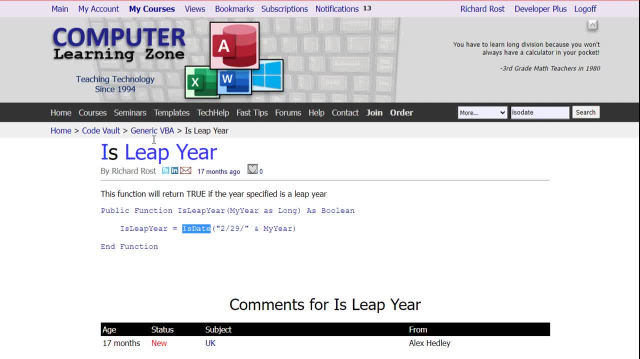 gold members. this is in the code vault. all right, you can go find it in the code vault. another reason why it's beneficial to join: there's all kinds of cool little functions like this floating around in here. if you want to learn more about this kind of stuff, i cover logical. 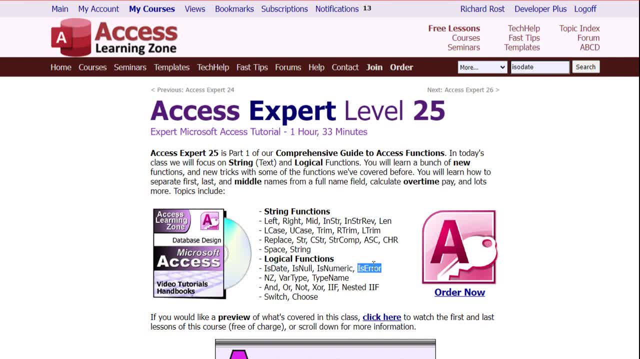 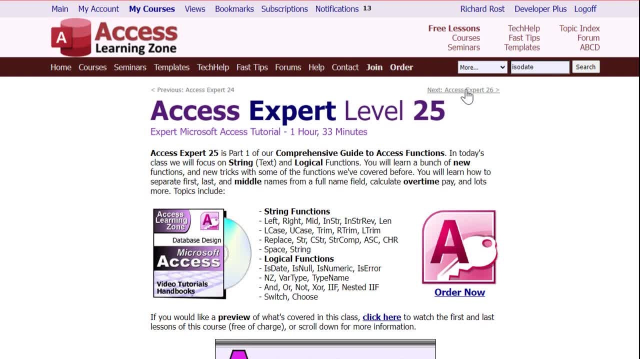 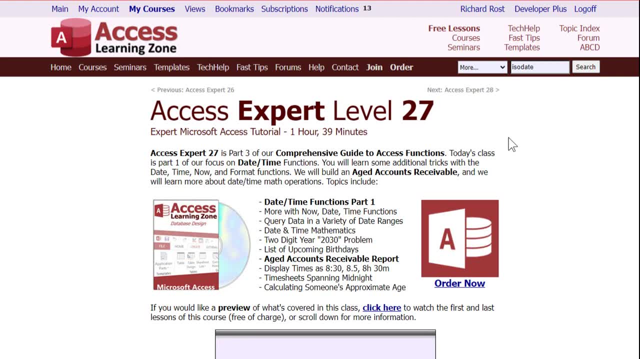 different functions apart. we go through the logical functions, we go through string functions, we go through the math functions, we go through the type conversion functions, date time functions. we go through all the functions over the course of a couple hours and i explain them all in detail. and that's one of the major reasons why you want to take my full course, because i cover things in. 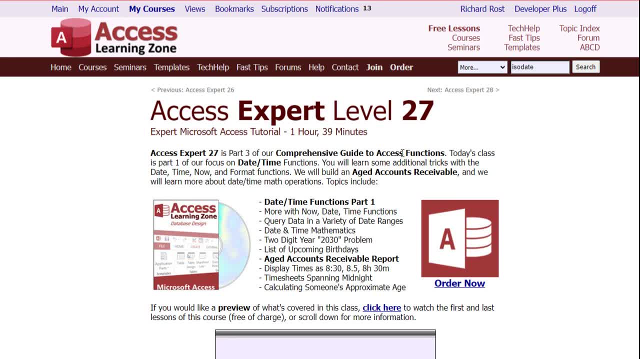 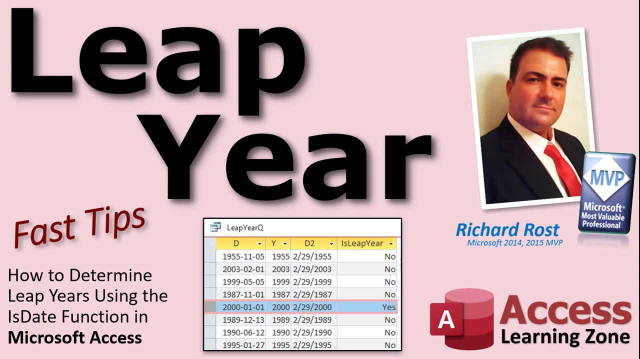 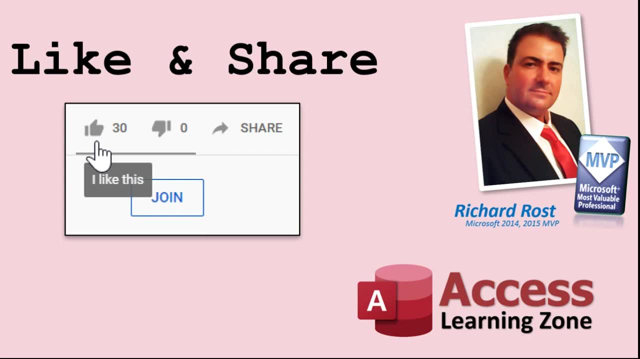 the order. you should learn them, not just randomly like i do with these fast tips. but that is your fast tip for today. i hope you learned something and we'll see you next time. if you enjoyed this video, please give me a thumbs up and post any comments you may have. i do try to read and answer all of them as soon as i can make sure you subscribe. 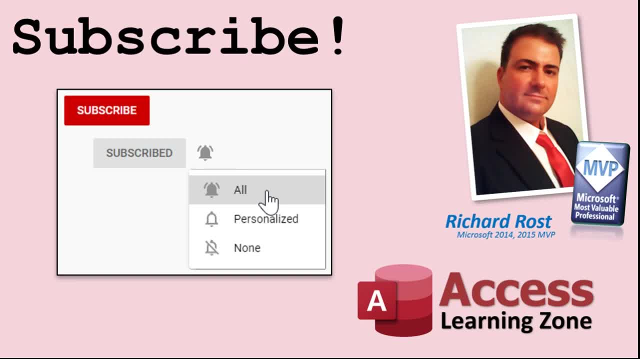 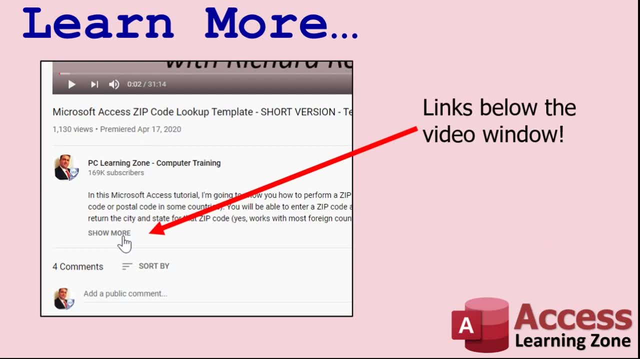 to my channel, which is completely free, and click on the bell icon to select all to receive notifications when new videos are posted. make sure you click the show more link down below the video to find additional resources and links. you'll see a list of other videos- additional information. 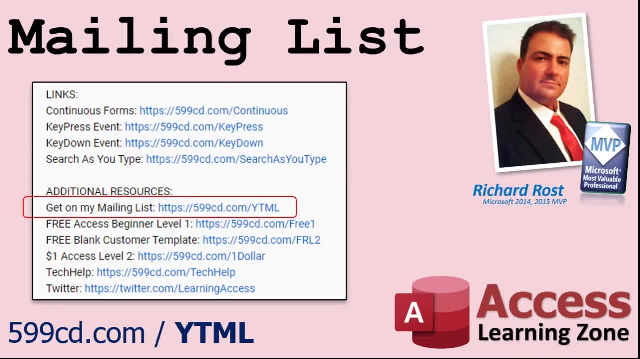 related to the current topic: free lessons and lots of other videos. i'll see you next time. youtube no longer sends out email notifications when new videos are posted, so if you'd like to get an email every time i post a video, click on the link to join my mailing list, even if you don't. 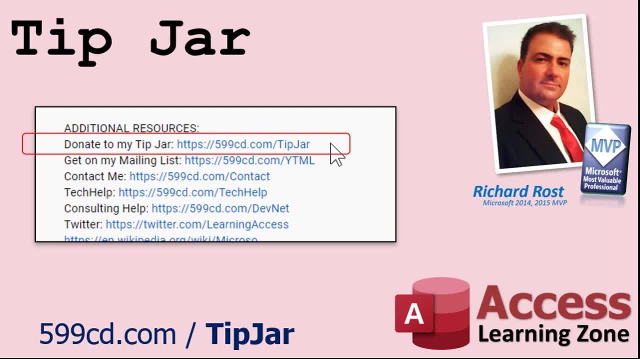 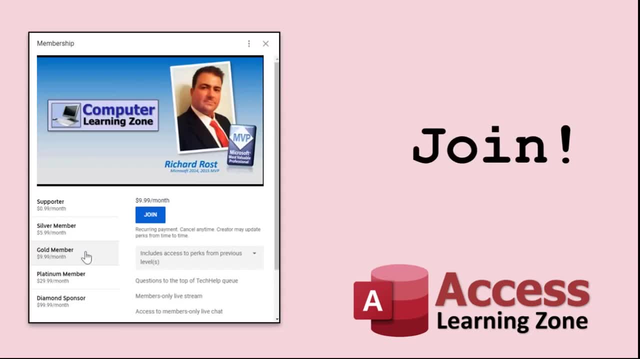 want to become a member, feel free to donate to my tip jar. your patronage is greatly appreciated and will help keep these free videos coming. i got puppies to feed. how do you become a member? click on the join button below the video. after you click the join button, you'll see a list of 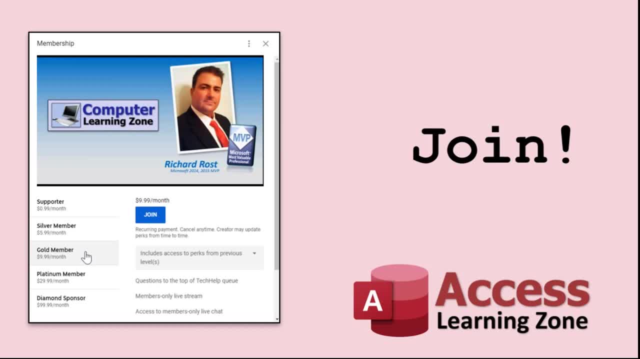 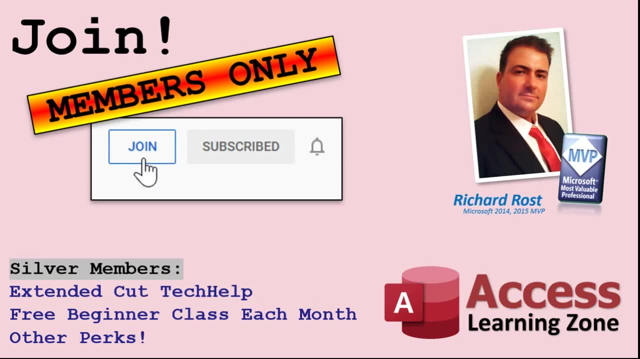 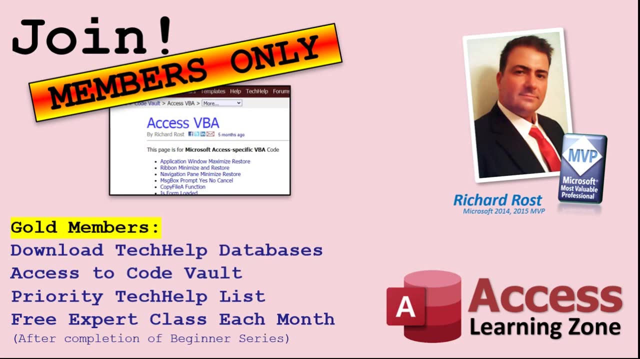 all the different membership levels that are available, each with its own speciality perks. silver members and up will get access to all of my extended cut tech help videos, one free beginner class each month and more. gold members get access to download all of the sample databases that i build in my tech help videos, plus my code vault where i keep tons of different. 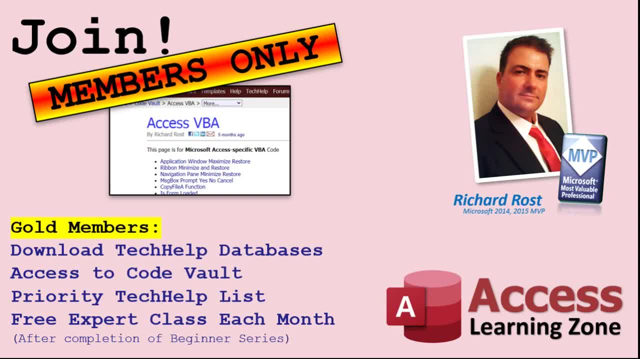 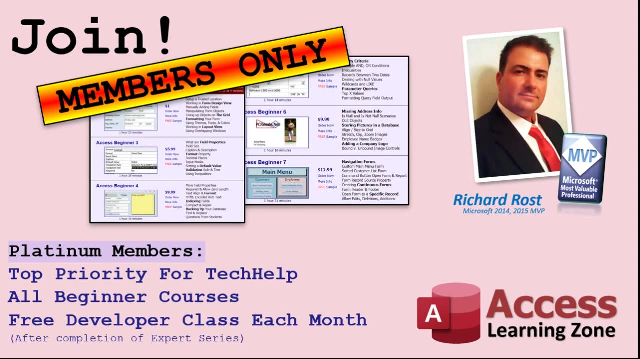 functions that i use. you'll also get a higher priority if you decide to submit any tech help questions to me, and you'll get one free expert class each month after you finish the beginner series. platinum members get all the previous perks plus even higher priority for tech help questions, access to all 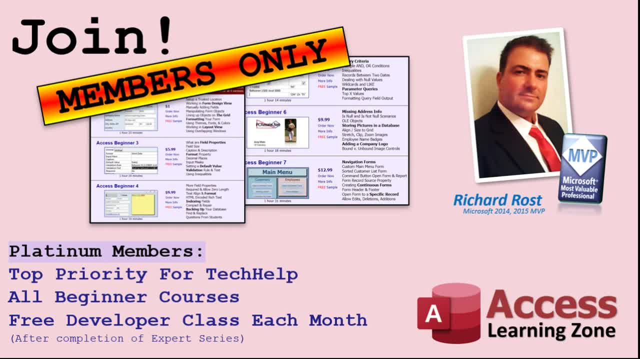 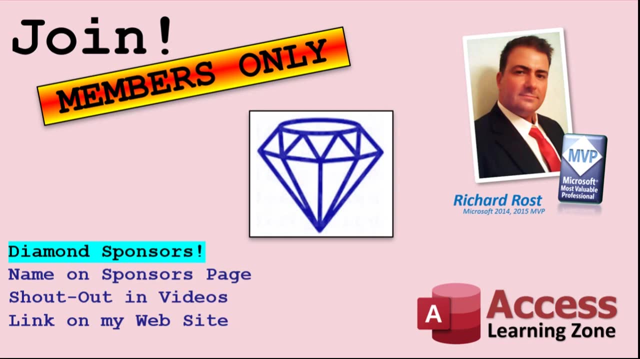 of my full beginner courses for every subject and one free developer class each month after you finish the expert classes. these are the full-length courses found on my website, not just for access to. i also teach word, excel, visual basic and lots more. you can now become a diamond sponsor and 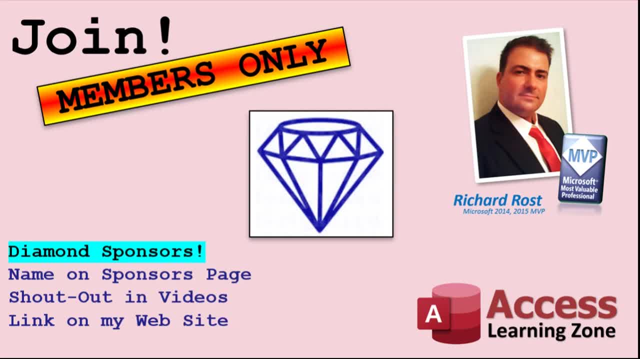 have your name or company name listed on a sponsors page that will be shown in each video. as long as you're a sponsor, you'll get a shout out in the video and a link to your website or product in the text below the video and on my 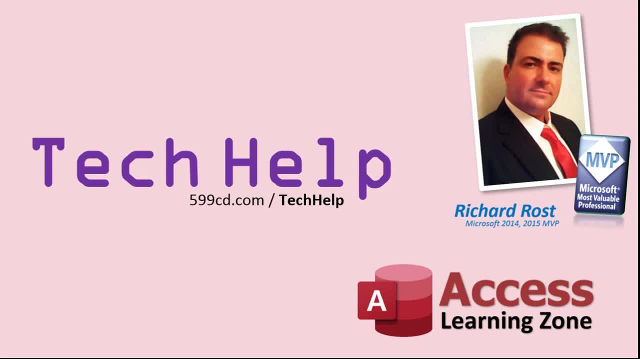 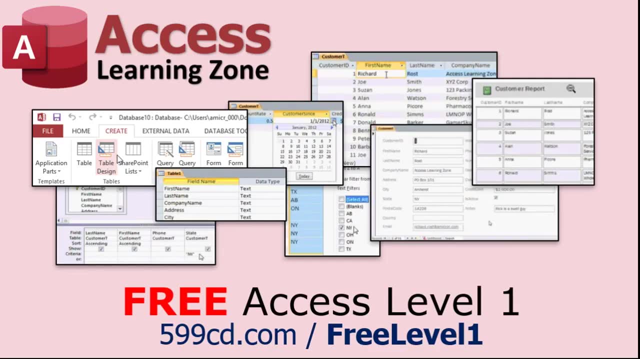 website. but don't worry, these free tech help videos are going to keep coming as long as you keep watching them. i'll keep making more and they'll always be free. now, if you have not yet tried my free access level 1 course, check it out now. it covers all the basics of Microsoft access. 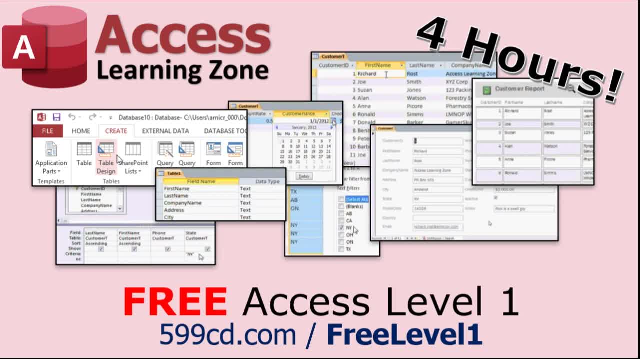 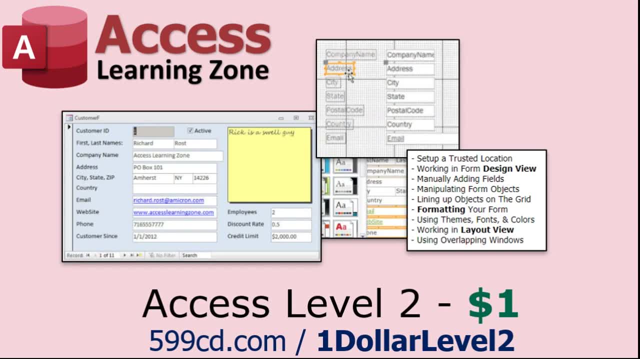 it's over four hours long and I just updated it for 2021. you can find it on my website or on my YouTube channel. I'll include a link below that you can click on and also, if you like, level one. level two is just one dollar. 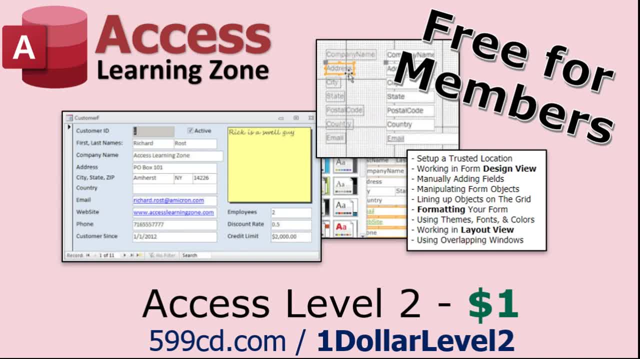 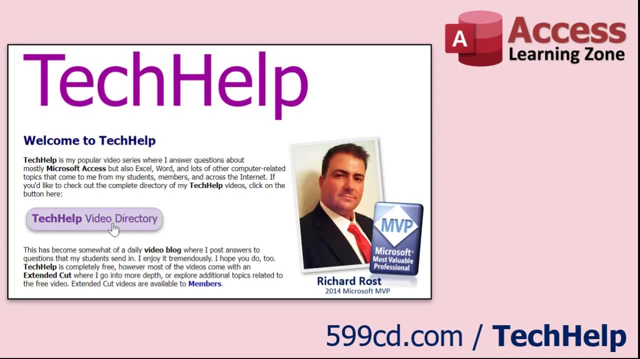 yep, that's all one dollar and it's free for all members of my YouTube channel at any level. even supporters want to have your question answered in a video just like this one. visit my tech help page on my website. you can send me your question there. while you're on my site, feel free to stop by the. 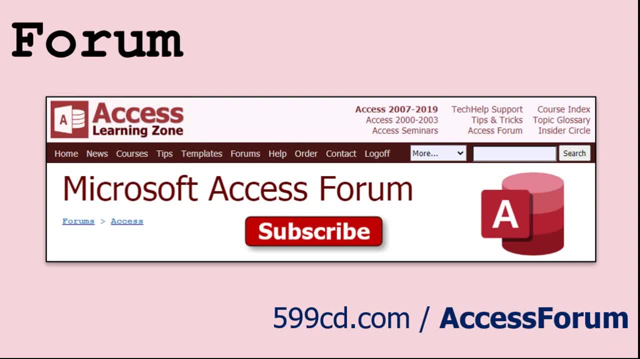 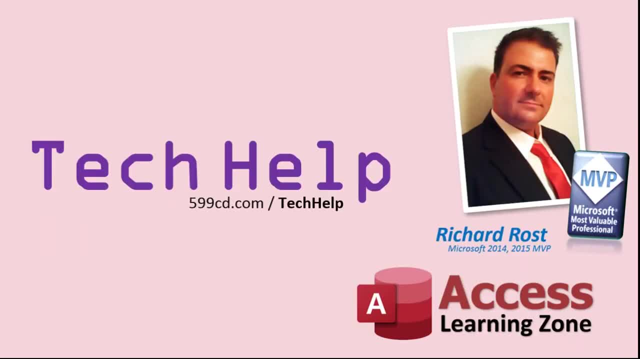 access Forum. lots of good conversations happening there. be sure to follow my blog, find me on Twitter and, of course, YouTube. once again, my name is Richard Ross. thank you for watching this tech help video brought to you by accesslearningzonecom. I hope you enjoyed this video and that you learned something today. I'll see you again soon. you. 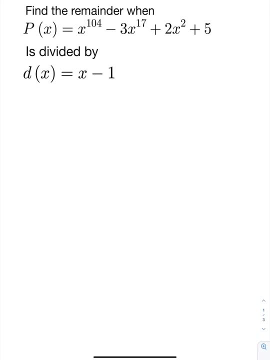 So we want to take a look at the following problem here. We want to find the remainder when we divide the following polynomial by x minus 1.. Now, if you remember the remainder theorem, the remainder theorem says that if a polynomial is evaluated at a real number, r, then that value. 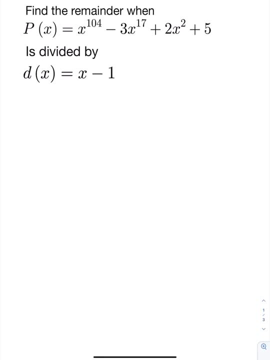 in this case p at r is the remainder when you divide that polynomial by x minus r. So using the remainder theorem here, we know that I can take my divisor here: x minus 1.. If I want to find out what the remainder becomes when I divide into the polynomial p at x, the only thing I need 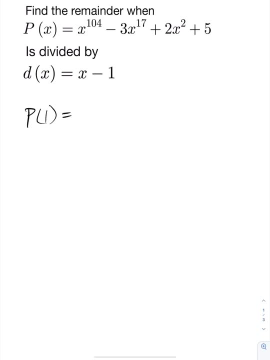 to do here is evaluate my polynomial at 1.. Doing so, we get 1 minus 3 plus 2 plus 5, and that'll simplify just to become a 5. So the polynomial at 1 is 5, and therefore, when p at x is divided, 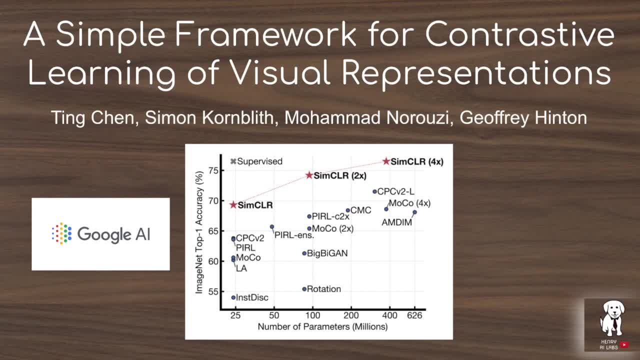 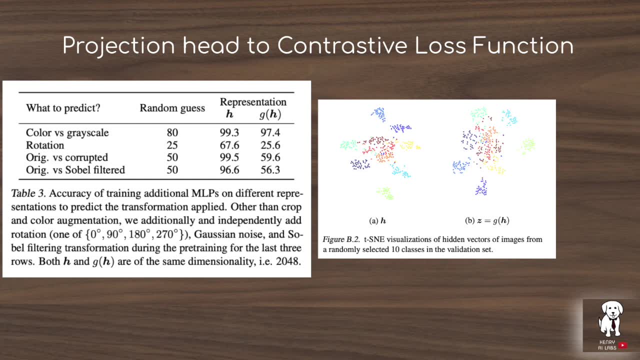 This video will explain the SimCLR algorithm from researchers at Google, which is the latest and greatest for unsupervised learning. SimCLR achieves the same performance as a ResNet50 trained with supervised learning on the same dataset, although this comes at the cost of. 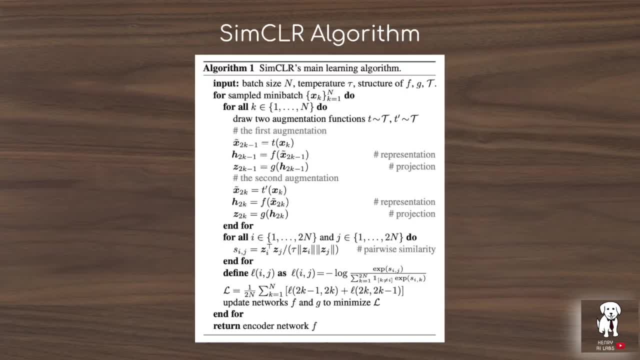 longer training time and larger networks. SimCLR uses contrastive self-supervised learning to leverage unlabeled datasets for representation learning. Self-supervised learning describes this idea of forming a supervised learning task automatically from unlabeled data, and contrastive learning describes the idea of training networks to have high